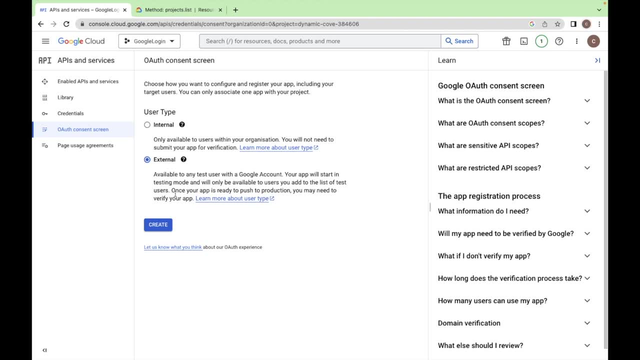 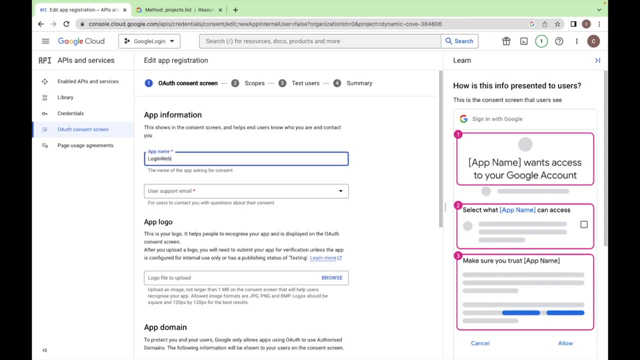 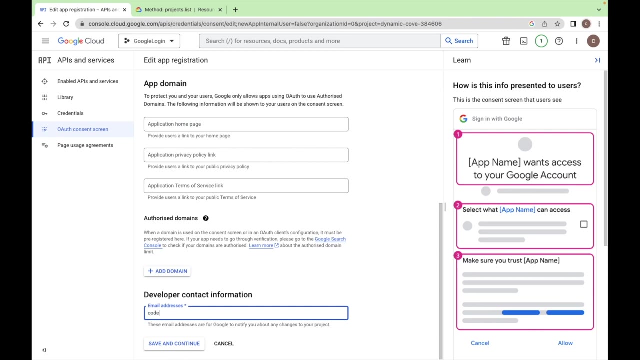 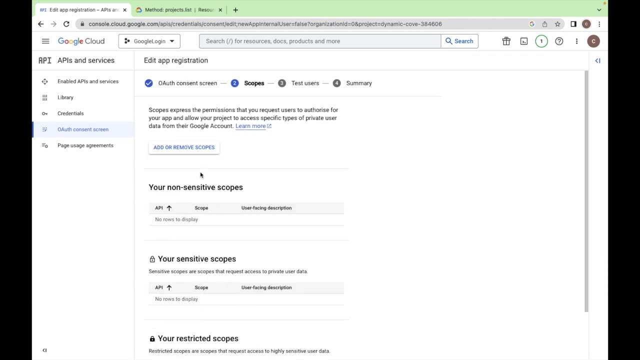 So you can test your app with the test users And click on create. Enter the app name, Login web. These are the optional fields, So enter the developer contact information, Save and continue. And next we have to add the scope. 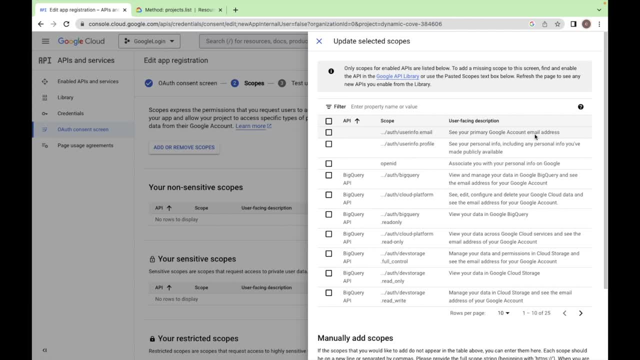 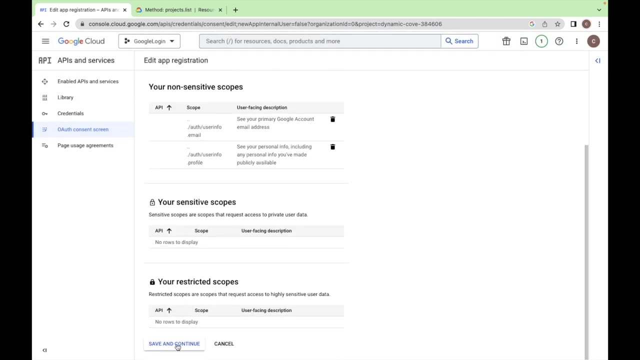 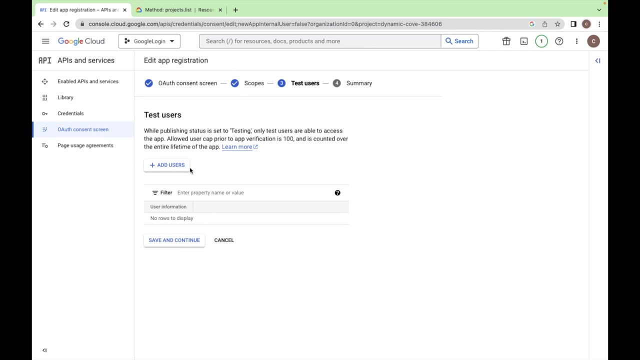 let's add two scope for now. see your primary Google account email address, select this option and see your personal information, including your personal info you have made public available. select this option also and update, click on save and continue. so add the user here, so by which you want to test this app, so 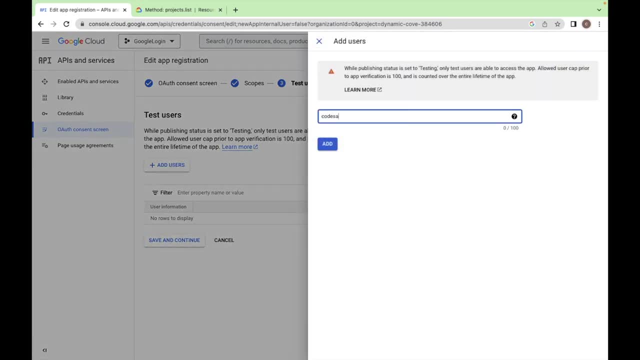 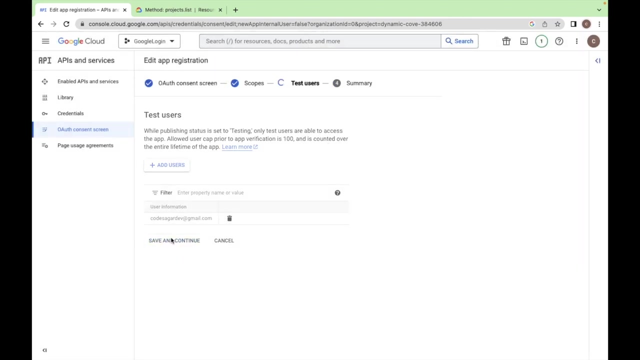 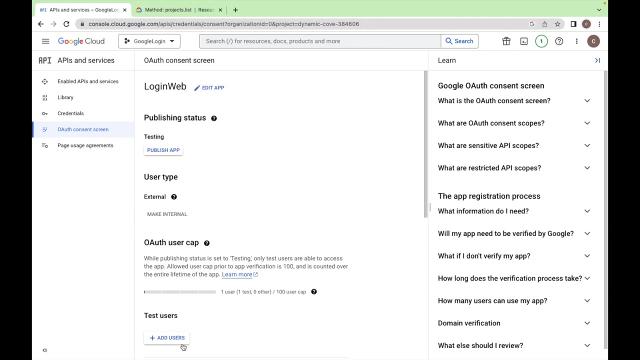 I want to test my app with the user code Sagar dev at gmailcom. add one and save and continue. this is the summary screen. back to dashboard. this app is in testing mode so we can test this app. so I want to test my app with the user code Sagar dev at gmailcom. add one and. 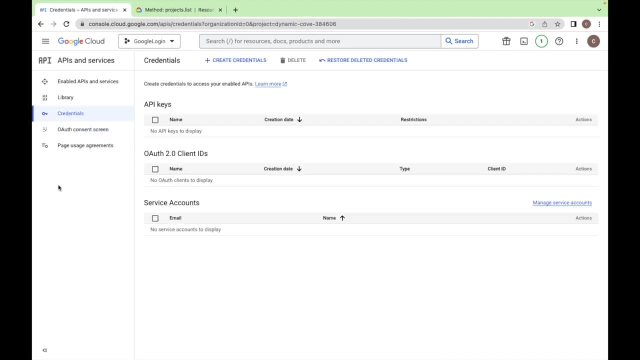 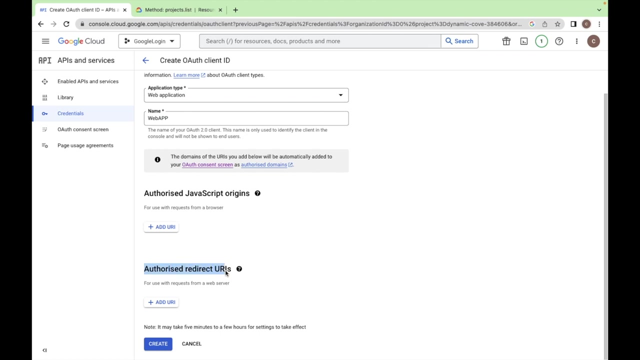 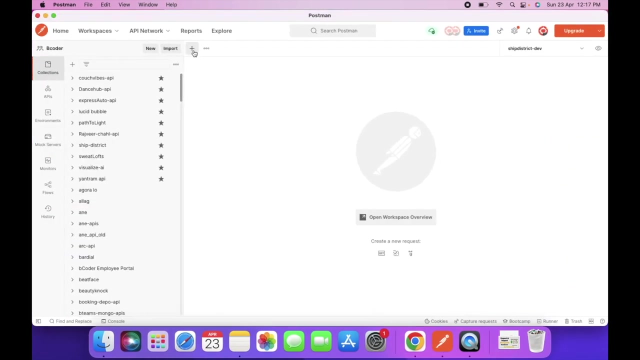 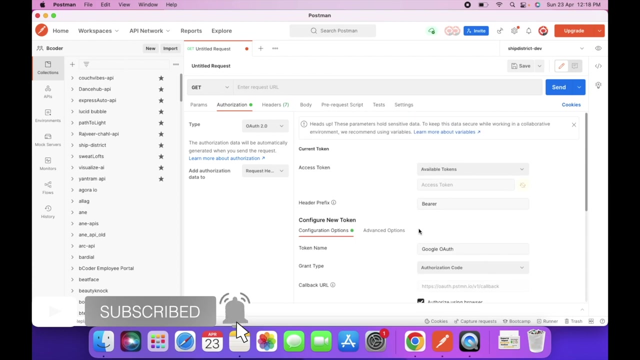 the test users. so click on the credentials and create one credentials. now select the web application type. this is web app. here we have to enter the redirect URL of postman. so go to postman and click on add. so go to the authorization tab and select OAuth 2.0. so here you have to select the. 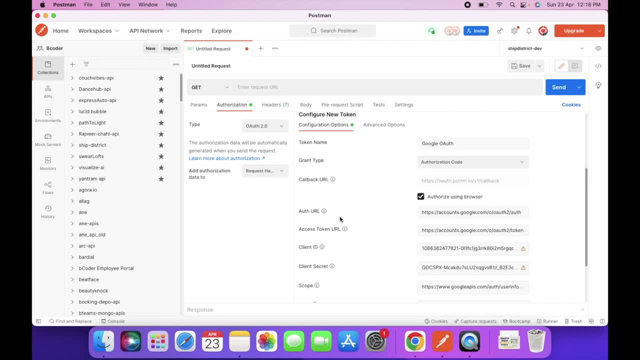 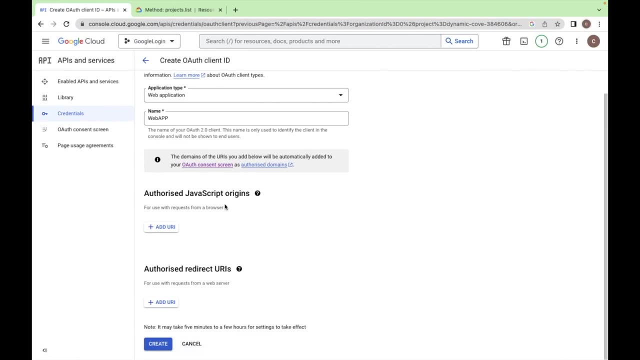 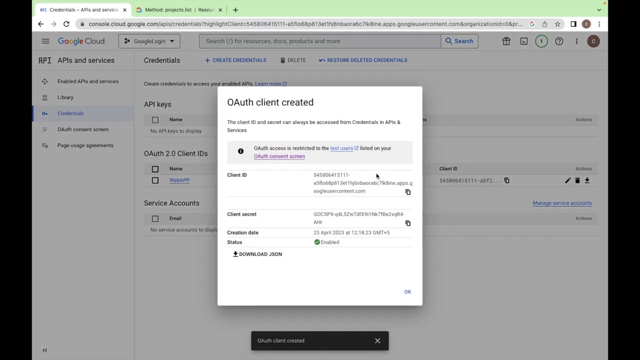 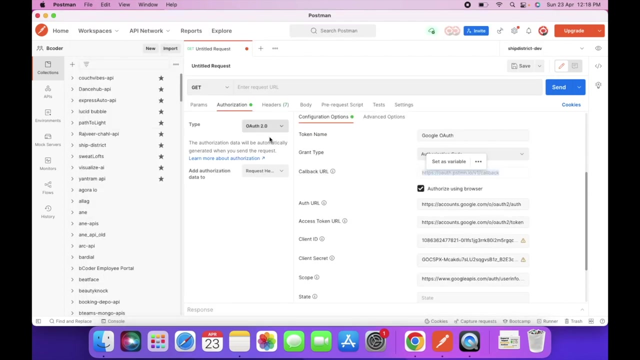 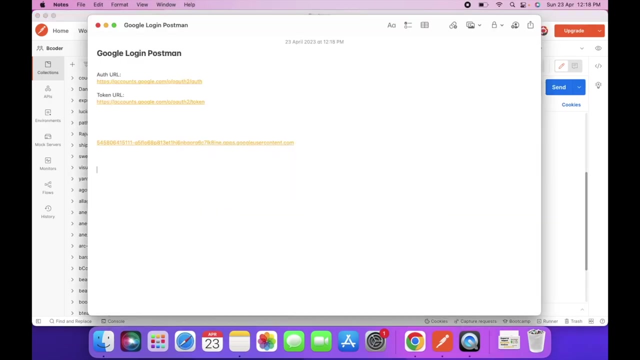 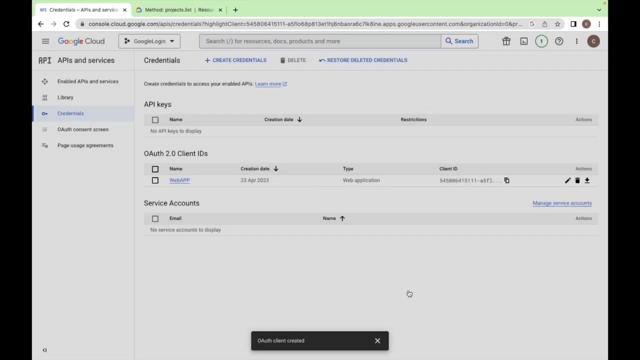 authorization code from the grant type and then you will get the redirect URL of postman. copy this URL, add URI and paste it here. click on create, so your credentials are created. copy this client ID and copy the secret key also, or you can download the JSON file also. click OK. so let's go to postman. 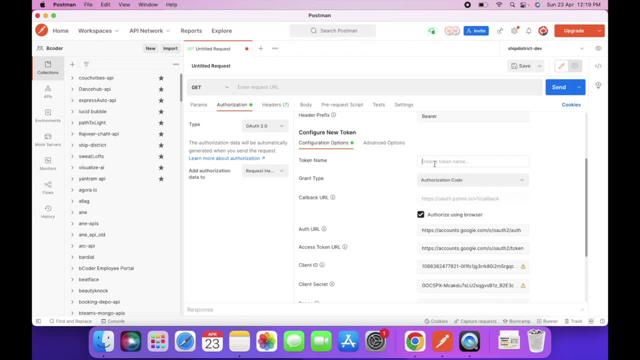 so here you can enter the name of token- so let's say codesaagr token- and select authorization code: authorize using browser. so I have already selected this option. so here you have to add the OAuth URL. so I will put these URLs into the description so you can check and 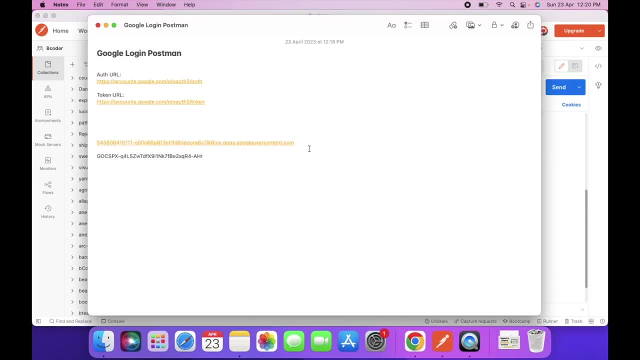 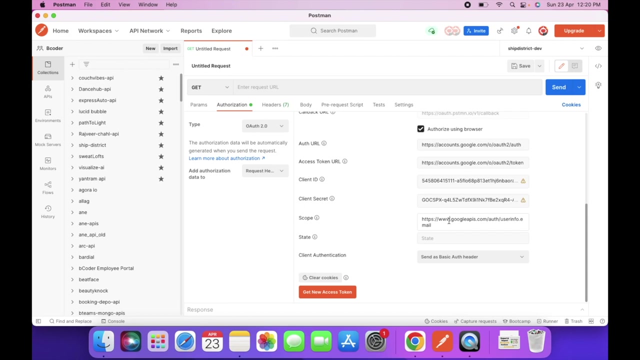 and here you have to enter the client id which we have just created. copy this id and paste it. and copy the secret key and paste it. here you have to add the scope. so right now i am adding only user info dot email scope. so next you have to click on the get a new access token. click on this. 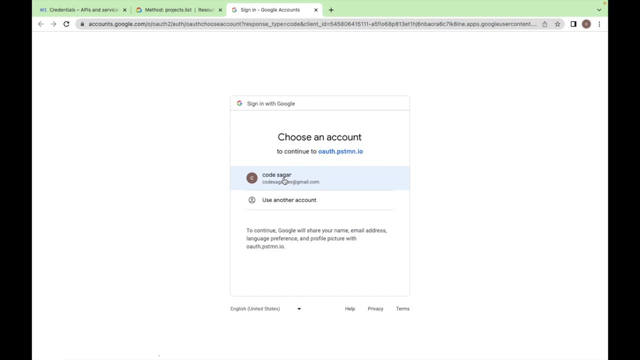 this will ask you to log in with the email id, so you have to log in with the id which you have put in the test users. let's log in with this email. so make sure you have enabled the pop-ups. so you have to go to the settings. 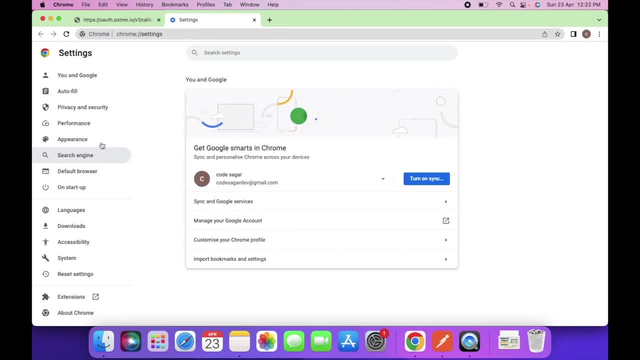 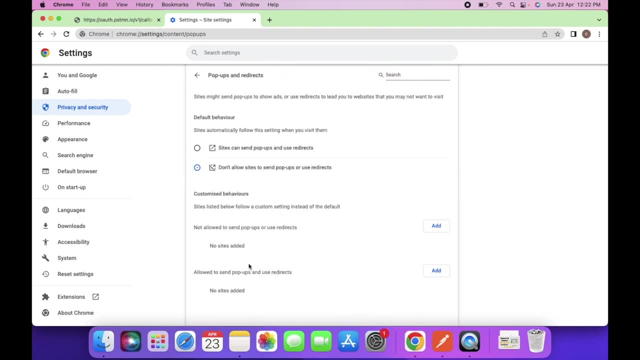 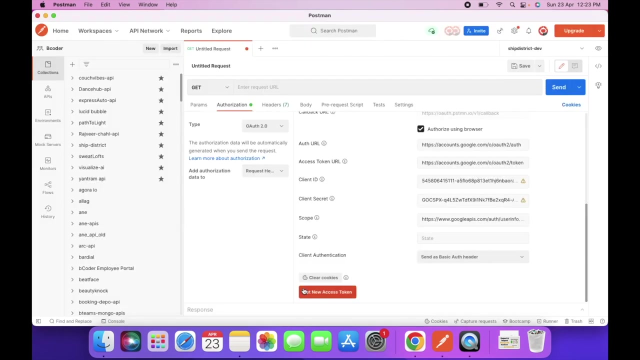 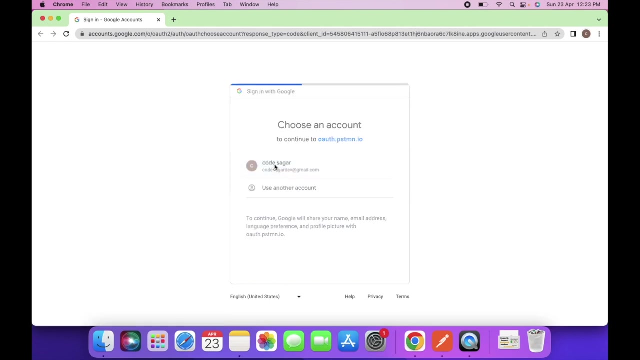 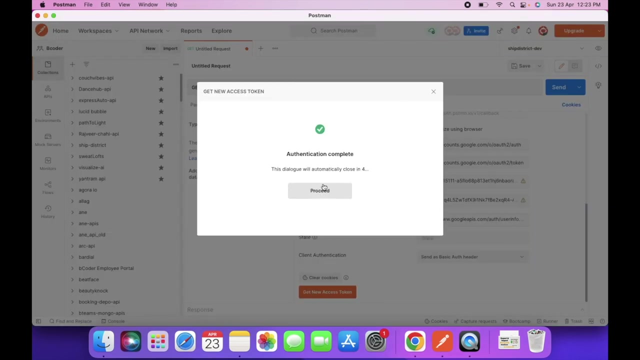 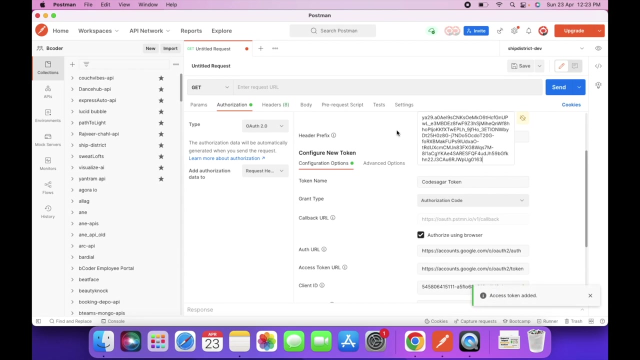 so privacy and security. click on site settings and pop-up and redirect. so select this option. sites can send pop-ups and use redirect back. let's retry to journey token so you can see open the postman. click on proceed and this is the token we have just generated. use this token so we are done with the. 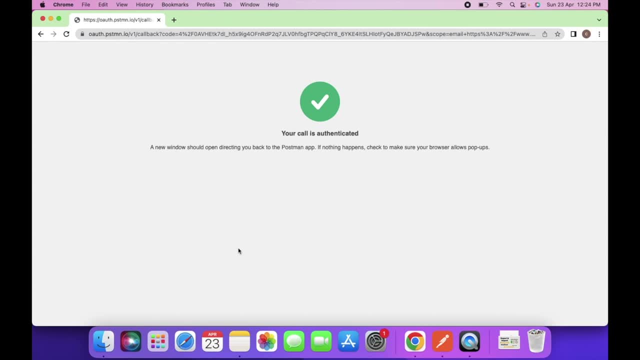 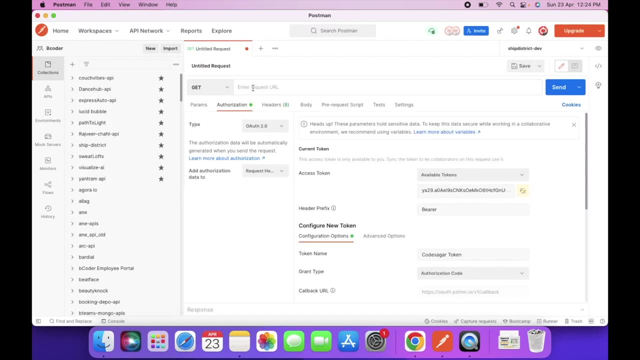 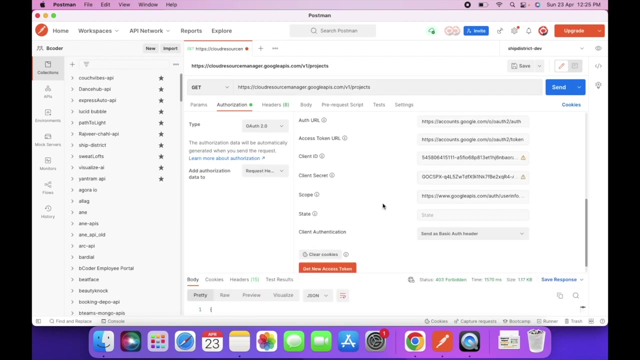 Google login. so let's try to fetch the projects in the cloud. to fetch the list of projects, we have to call this URL, enter this URL. so, as you can see, request had insufficient authentication scopes. we have to add one of the scope. copy this scope and enter here. to add multiple scope in one request, just enter. 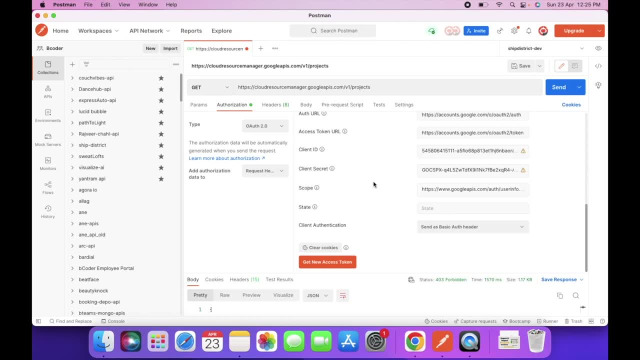 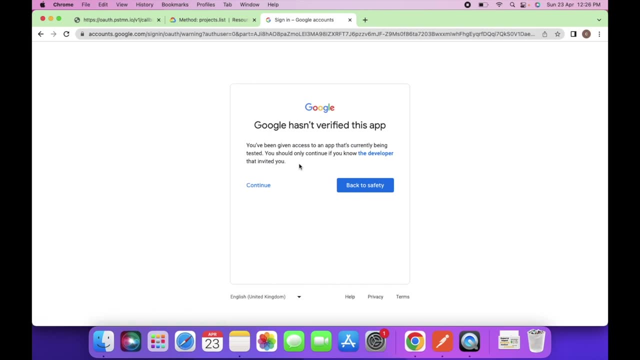 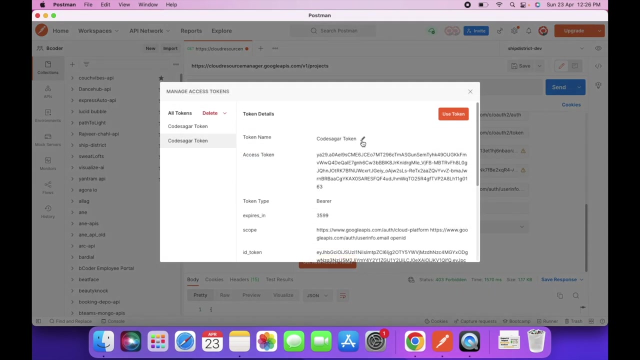 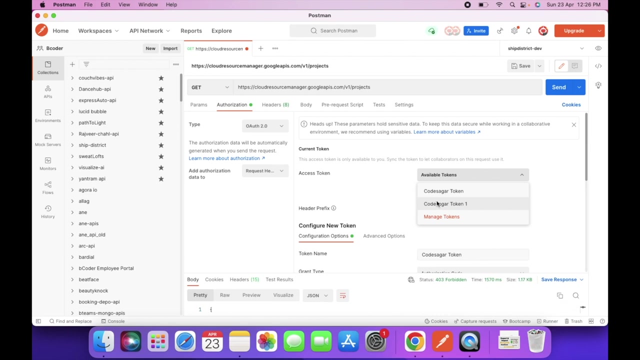 space and paste to the another scope. so let's create a new access token and so this will ask for the permissions. click on continue. so this will ask for the cloud permissions. continue and open postman. go to proceed. we name it token one. so we have to select that only test token here and click on send. 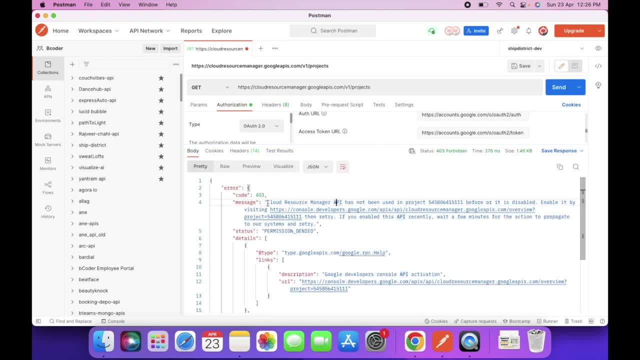 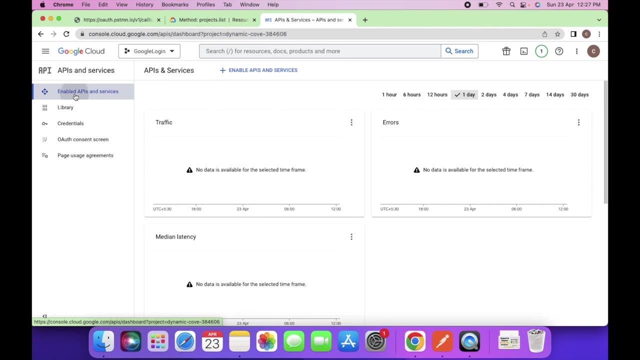 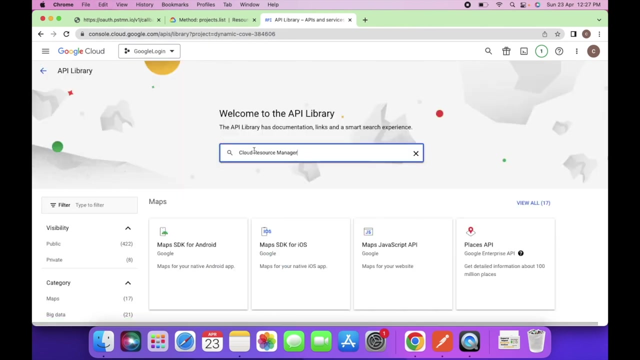 pressing ok and now we are done for today's session. we are finished here, so now we are getting this error. cloud or source manager API is not enabled. currently, this is the disabled, so let's enable thisAnother source of nature API from the project. click on enabled API services. click on this add button and.